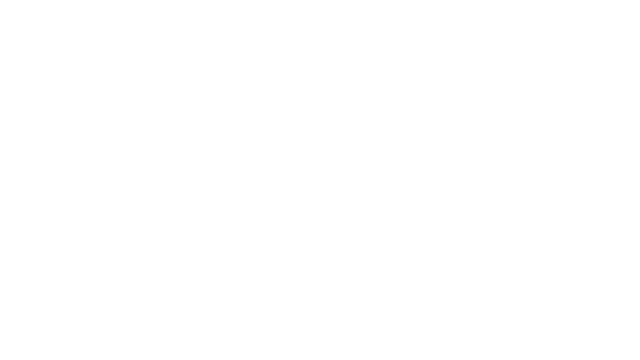 in this video I'm gonna teach you how to solve mean, median and mode of a group data. so let's take, for example, we have this, a table where it composed of an age from 10 to 24 and it is grouped by three from first column we have from: 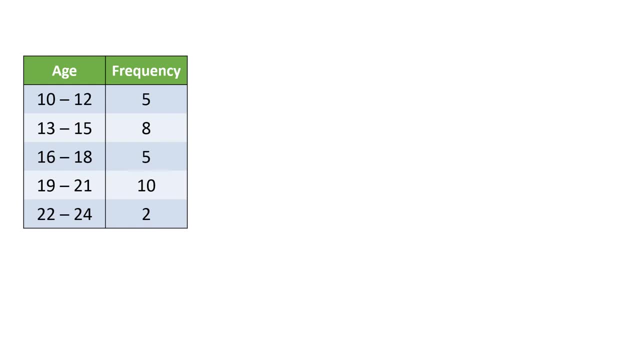 ages 10 to 12. that means it's 10, 11, 12 and there are five in the frequency it means there are five, five participants ranging from 10 to 10 to 12 years old. but we don't have an idea which of these are these five? either there are five tens, or some are 10, some 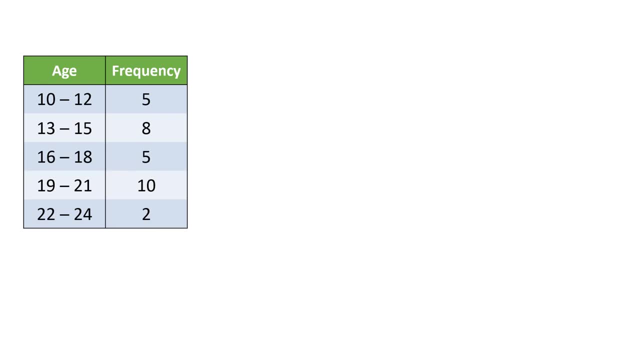 are 12, some are 11, so we don't know, but we are sure that these five are just within the range of 10 to 12, same as from 13 to 15 years old. there are 8. 16 to 18 years old. there are 5. 19 to 21 years old. there are 10 and 22 to 24 years old. 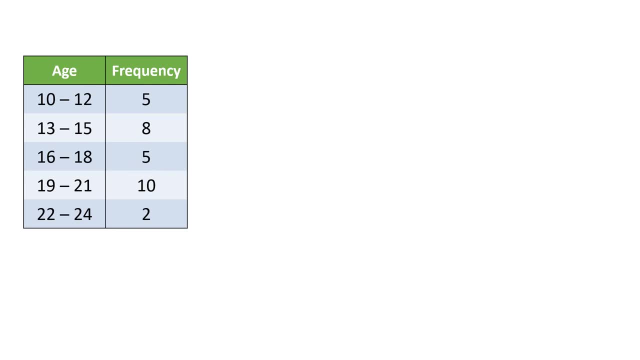 there are 2 participants. so that is what you call the group data. so you really have no idea what is the exact data or age, but you have only the idea by grouped, and we want to know how to solve the mean. so we're gonna find the mean and finding the 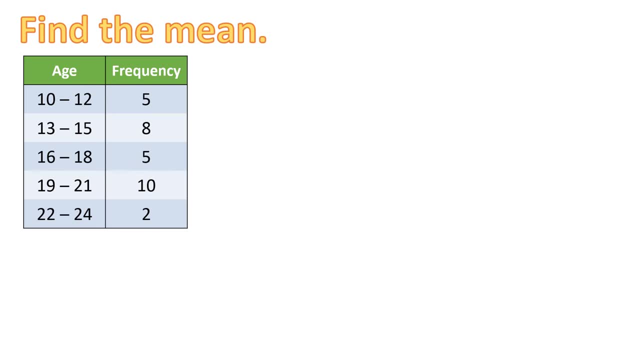 mean of a group. data is totally different, finding the mean of a group. so we follow a formula for the mean. so we have this symbol for the mean and X bar which is equal to the sum of FX. so this, the Sigma symbol before the FX, is what you call the summation. it means the 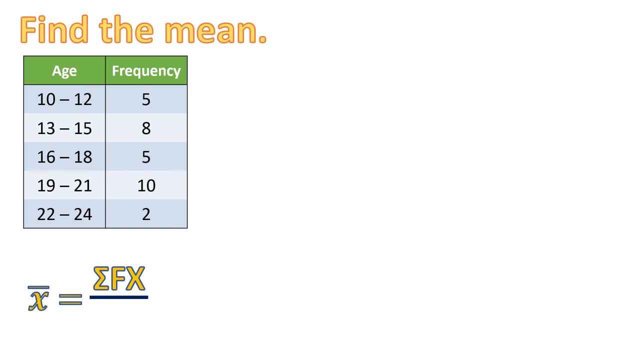 total, or the sum of the product of F and X, and you will know later what is that X divided by n and is the total frequency. so, based on the formula, we need the to add a column, a column for X. so what is that X column? so X is actually the class mark. 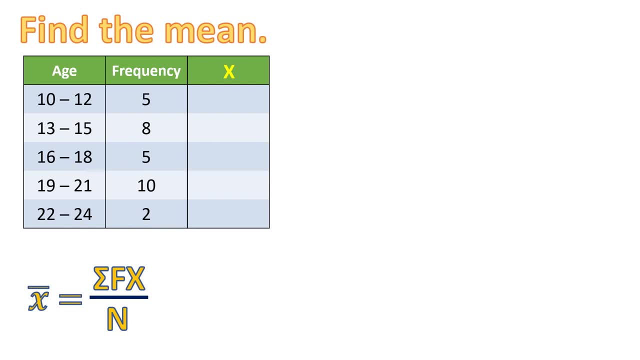 so sometimes we put CM as class mark or or X, but for me I I'm used to use X instead of CM, since it's only one letter and class mark, or the X is actually the middle number of the interval from 10 to 12. what? 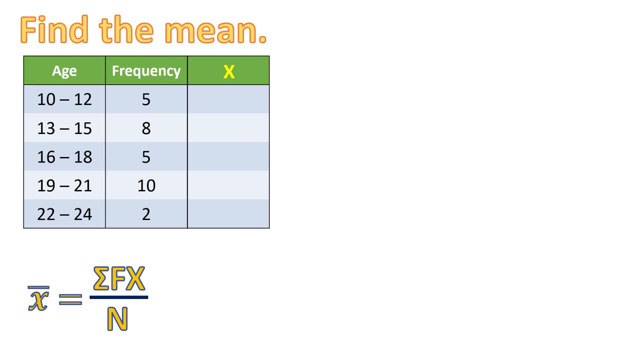 is the middle of that: 13, 15 and so on. or you can just add 10, 12 divided by 2. that's the shortcut, finding the middle number, that's the middle number and the value of an interval. so anyway, this is only three, uh, an interval of three, ten, eleven, twelve. so 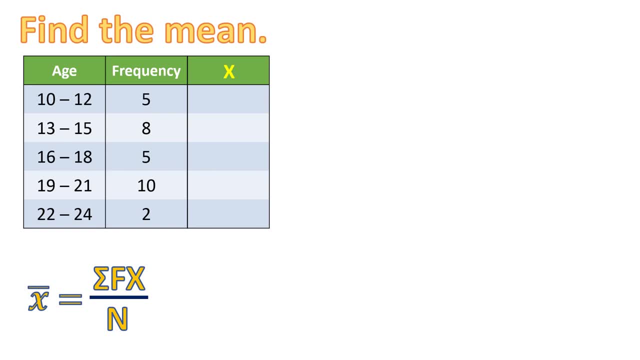 obviously the. the class mark of the first row is 11, because that's the middle, or you can add: 10 plus 12 is 22, divided by 2 is 11. then the next one is in between 13 and 15 is 14 in between 16. 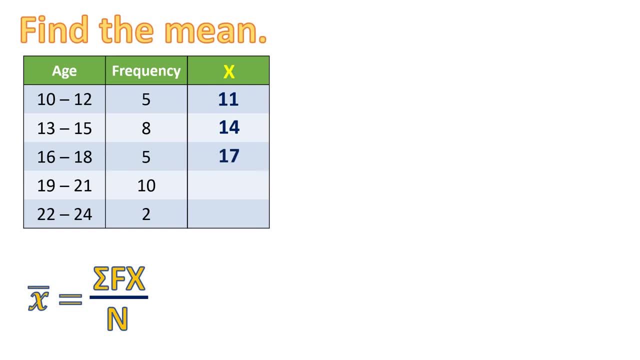 and 18 is 17, and then in between 19 and 21 is 20 and in between 22 and 24 is 23. so those are exactly in the middle of each interval. that is what you call the class mark. so after getting the class, 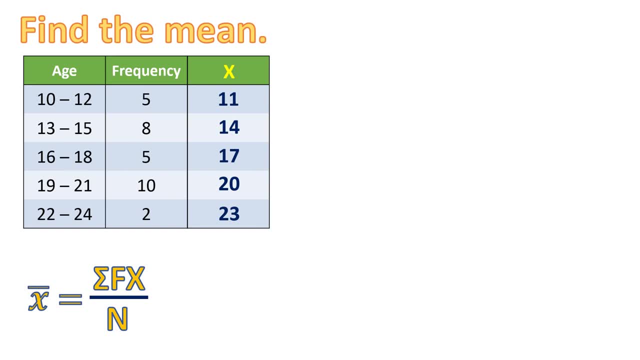 mark. we will need another column where we need to multiply the frequency and the x or the class mark. that's why the formula there is FX, because it's frequency times the class mark, so we will name it FX or the frequency times the class mark. so obviously it means we multiply the frequency. 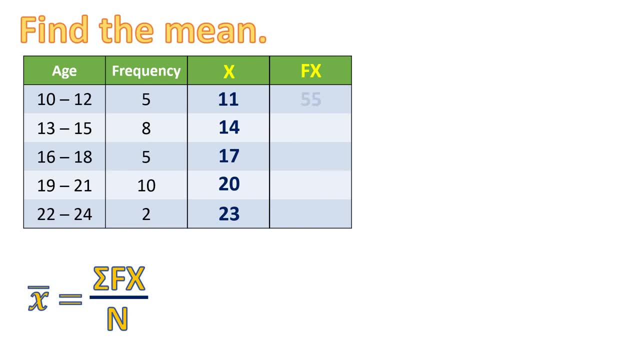 in the class mark. so it's: 5 times 11, 55, 8 times 14, 112, 5 times 17, 85, 10 times 20 is 200 and 2 times 23 is 46, and so, after completing the table, this is the columns. 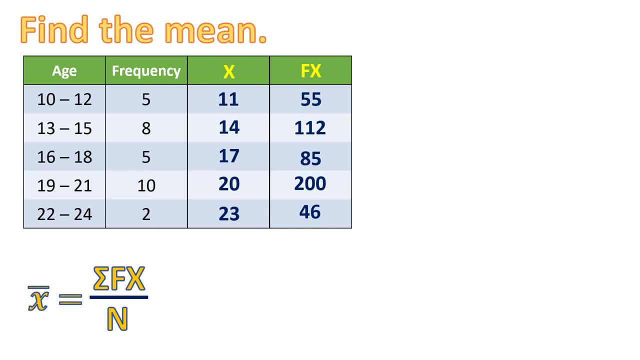 that we needed for finding the mean, the X and the FX. then we will find the sum, the sum of what? so we based on the formula which is sum of FX, so we will get the total of FX. so we add all 55 plus 112, up to 46, so the sum of FX is equal to 498, if you will use your calculator. 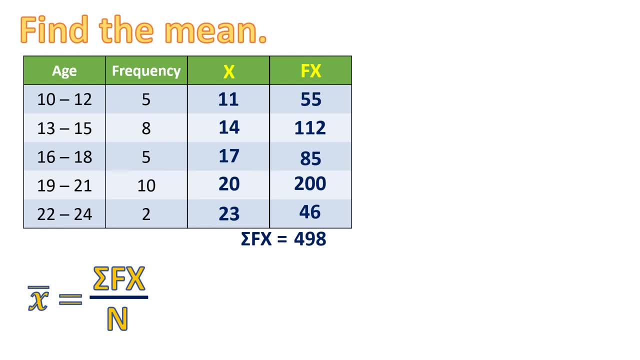 and so. so we have the sum of FX and then we still need capital N. so sometimes we put their sum of F because and it's actually the total frequency of the sum of FX, so we add all 55 plus 112, up to 46 for the sum of the frequency. so we'll solve for the end, which is equal to will. 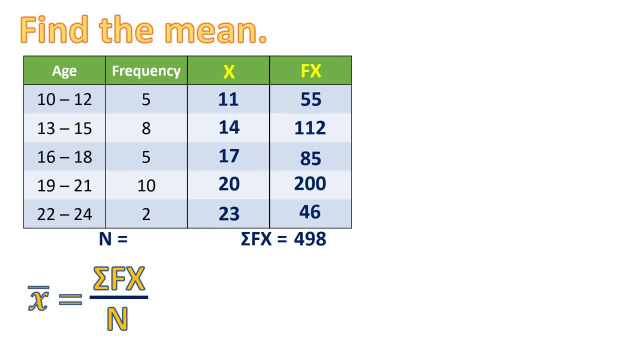 add all five plus eight plus five plus ten plus two is 30, so we will substitute these all 498 divided by 30. if you use your calculator, you will get sixteen point sixty and that's the mean or meaning. that's the middle uh age based on the given group data. 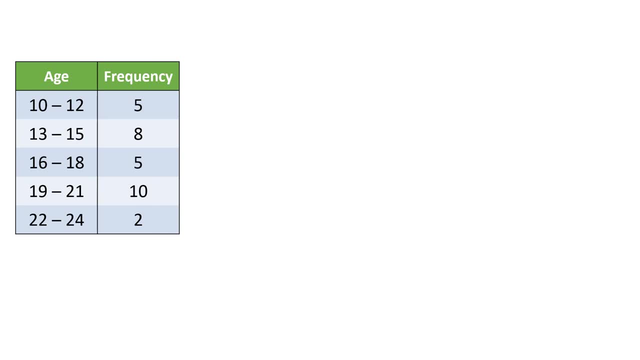 all right, so let us reset the given and then we're gonna find, uh, another one site for me. we're gonna find the median. so median is still finding the center. but you remember, in finding the median of what group data is to arrange them. but this time this is grouped and you don't need to arrange them because it's. 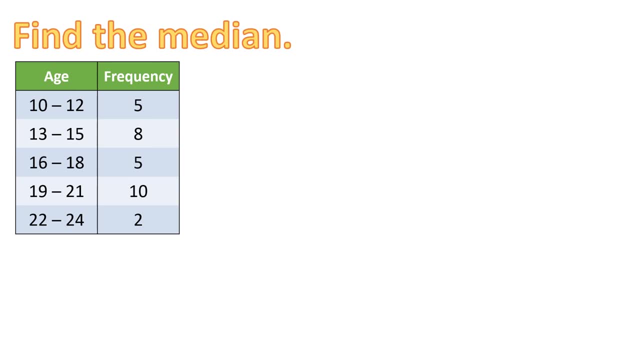 already arranged in a table, and so they are mean and median are computed differently, but uh, in most cases they that the results are almost uh similar for group data. so let me show you the formula to find the median. so median is written in this way: x wiggle. 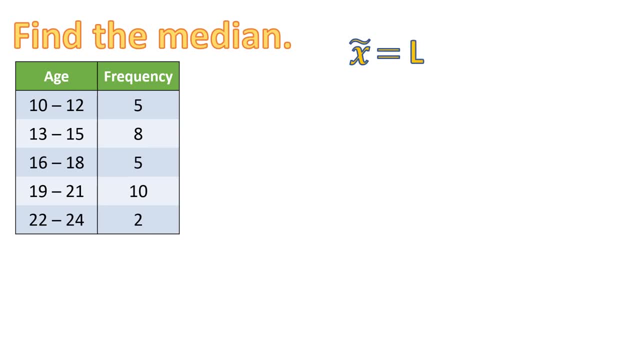 which is equal to uh. l stands for lower class boundary plus, so we need to put this: symbols, parenthesis and event column, and n, which is the total frequency divided by two minus the lower, less than cumulative frequency. so the l in the subscript means the lower or a lesser value less than cumulative. 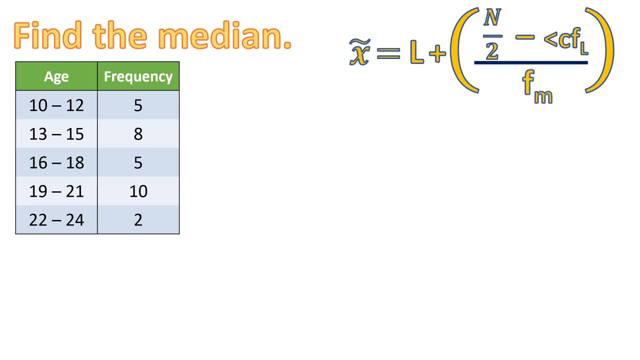 frequency, so all over the fm, or the frequency of the median class times, the class interval. so, based on the formula, we need the l, which is the lower class boundary, so we need that column, so we'll name it lcb or the lower class boundary, so lower class boundary is just simple to get. 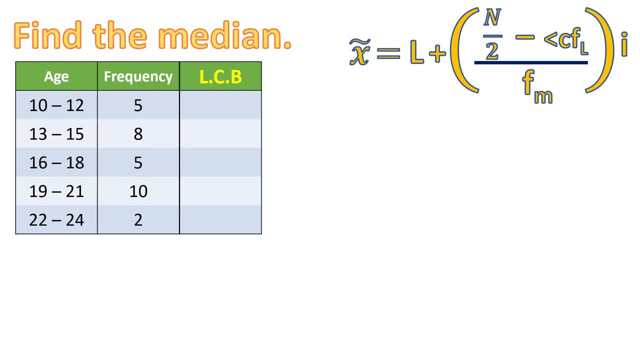 we subtract 0.5 to the lower limits in the interval. so lower limits are those numbers as small as numbers for each interval: 10, 13, 16, 19, 22. so we subtract 0.5 for each lower limit to get the lower class boundary for each. 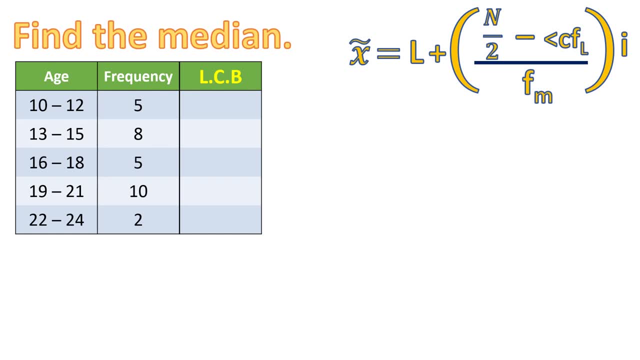 row. so for example we have: 10 minus 0.5 is 9.5, 12.5, 13 minus 0.5 is 12.5, 16 minus 0.5 is 15.5, 19 minus 0.5 is 18.5 and 22 minus 0.5 is. 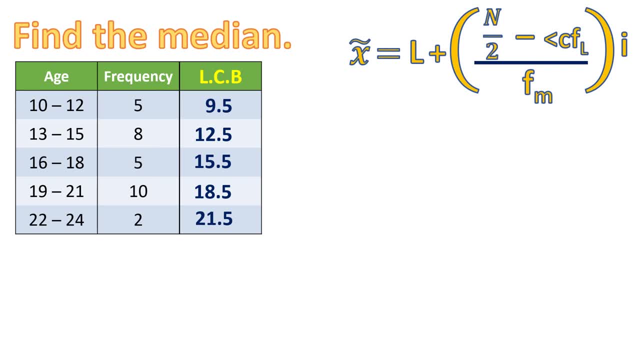 21.5. so that's lower class boundary, and that's how we say. it is now one more column that we needed, based on the lower class boundary, and that's how we say. it is now one more column that we needed, based on the lower class boundary, and that's how we say. it is now one more column that we need. 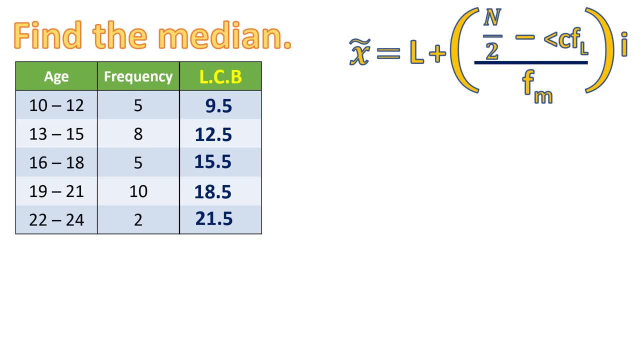 the formula is the less than cumulative frequency, so we'll add one more column and then we'll name it less than cumulative frequency. so there are two cumulative frequencies where there's less than, there's greater than community. but you don't need a greater than in this formula, so we'll use less than. 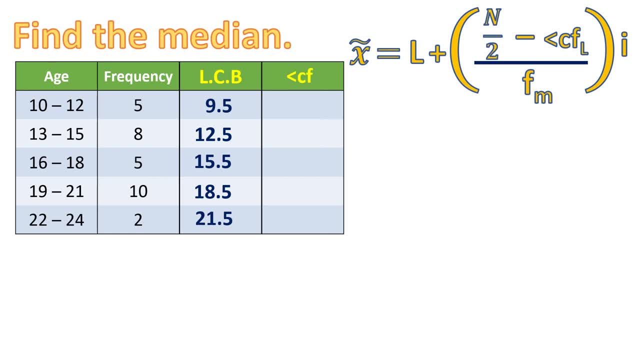 cumulative frequency. so less than starting from the smallest interval going to the biggest interval. well, the greater than is the other way. but you don't need it. so let's have the less than cumulative frequency. we we base our values of this column from the frequency. so for the first row of the less than cumulative frequency, we just 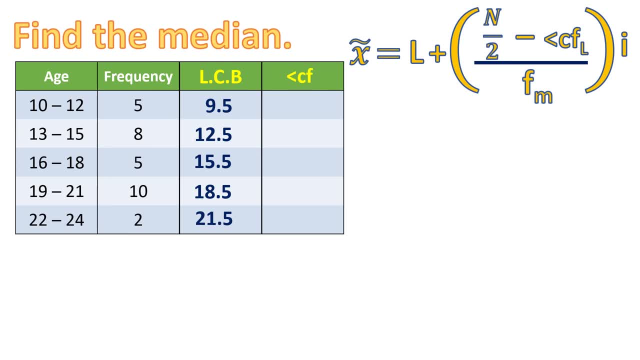 copy the frequency from the topmost row, which is five, and then what we do with this five is we're gonna add it to the next frequency. five plus eight is thirteen, then thirteen plus five, that's eighteen. and then eighteen plus ten is twenty eight. twenty eight plus two is thirty, so this is less than. 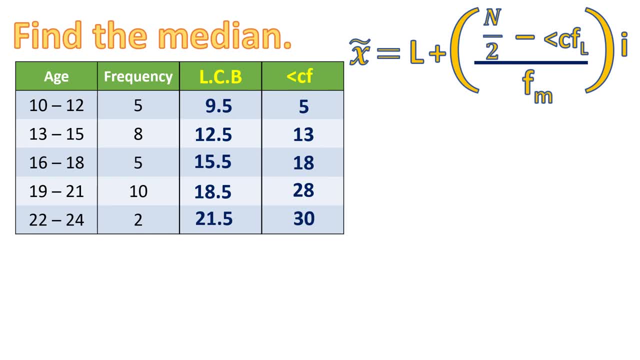 cumulative frequency. now, since we have completed our column, our table, then we can, we can substitute to our formula, but then we have a lot of lower class boundary, so which of these are we going to use? and there are also many less than cumulative frequency, so that means we need to know which row are we going to use. and there 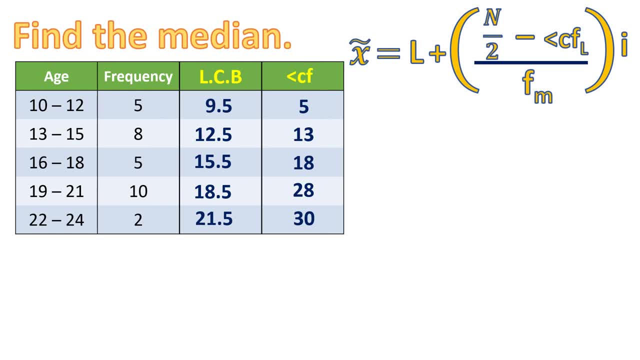 is a formula to follow to find this row, and this row is what you call the median class. so we will write it in this way: the median, with a subscript C indicating that it is the median class. so it's equal to the half of the total frequency. so total frequency, or the n is equal to. we'll add it all where we have that. 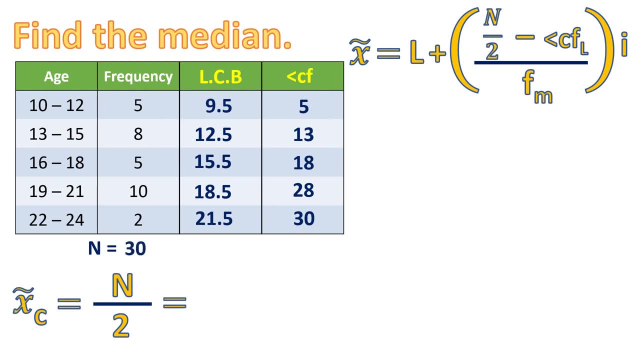 in the previous slide it is thirty. so half of thirty is equal to fifteen. but this is not yet the median. it's the median class, meaning it's the position. so we'll put the position symbol, which is th, which means it's fifteen, so the median class. 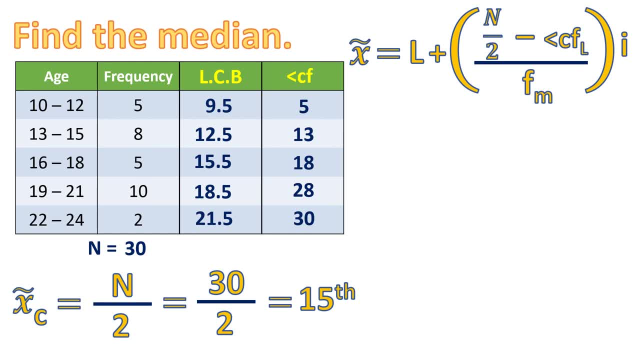 is located in the fifteenth position. now we're gonna look at the less than cumulative frequency and we're gonna find fifteen. so if there's no exactly fifteen, then we will find the closest number to fifteen above it. so fifteen is in between thirteen and eighteen and we always choose the bigger one. so the median class or the row that we need to use is the one 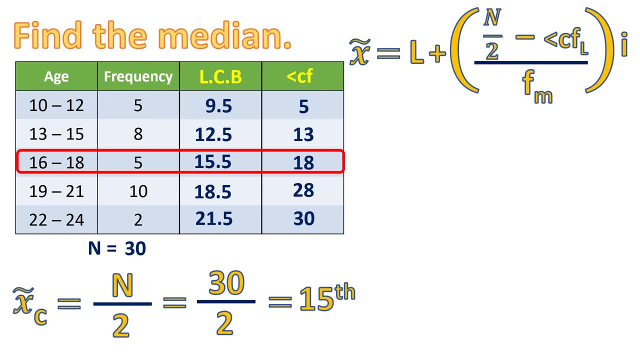 with the value of eighteen less than sia. so this is what you call the median class, and those values are the one that you're going to substitute with the median class, and that's what we're going to do, which is in the formula, except for the eighteen, and you will understand that later. 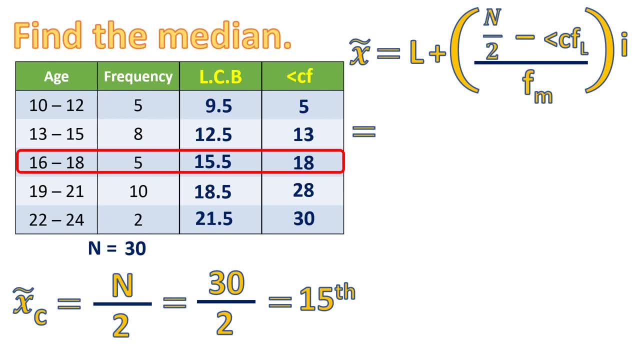 So let's continue. substitute: the lower class boundary is fifteen point five plus. so let's put those symbols, parenthesis and the venculun, and then we'll move to n over two. so n over two is actually the median class, where we have that which is fifteen fifteen. 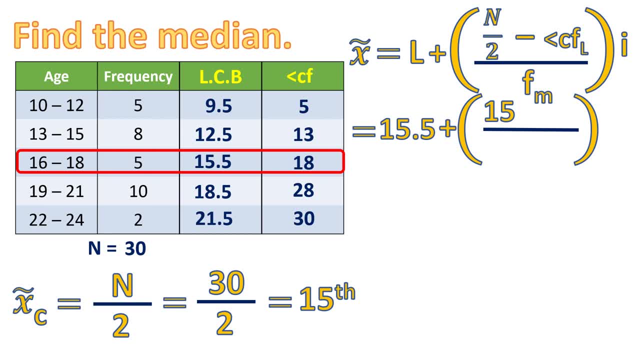 But we include the th because we just need the value 15 minus. now it's the lower, less than cf. so it's not the 18 that we will put, but it's the lower value. lower than that is 13. so it's 13 and then over. 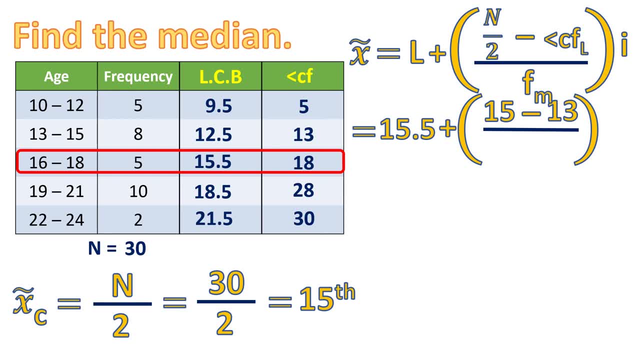 the frequency of the median class, which is 5 times the interval. so the interval is the same for all the rows. it's always. it's also. it's always 3. so 10 to 12, 13 to 15. so there are three numbers for each row for each interval. so let us continue solving. we are done. substituting. 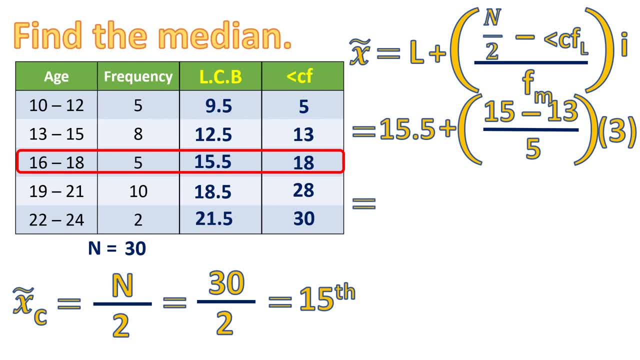 and let's compute. so let's uh, copy first the 15.5, because we cannot compute it yet. we will solve from the inside of the parenthesis. so copy the plus and we will solve from the inside of the parenthesis. so copy the plus and we will solve from the inside. 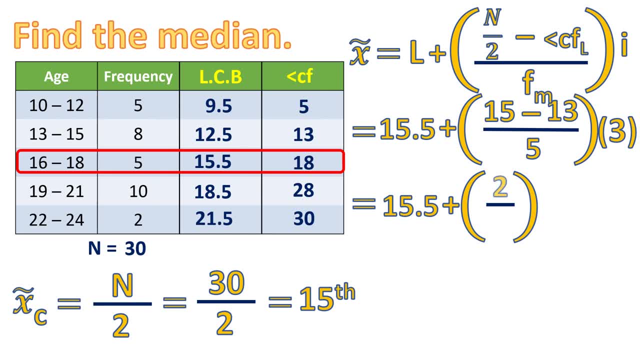 then let's solve: 15 minus 13 is 2.. Copy the 5 and 3.. So we will continue solving. Let's still copy 15.5 and plus, because we will just use it later And then we will decide here. 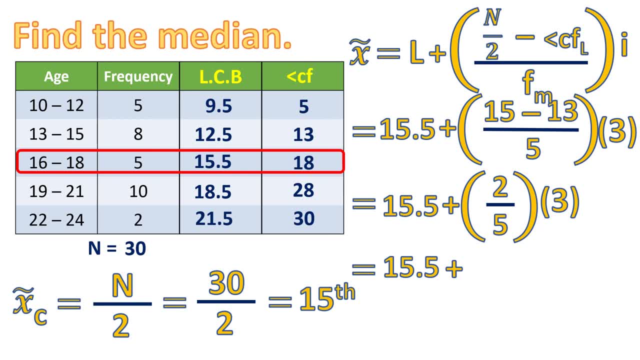 in this point, 2 fifths times 3.. So there are two ways to solve this. Either you do divide first, 2 divided by 5, and then you times 3.. Or you times 3, first, 2 times 3, and then. 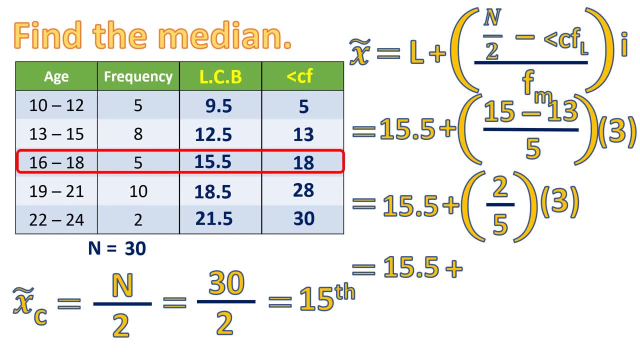 you divide by 5. So it's going to be the same result in this case, But usually you will have some problems when you divide first, then you times, because, like having a repetition in the decimal, So it's non-terminating, usually when dividing a number by a multiple of 3.. So to avoid complications, 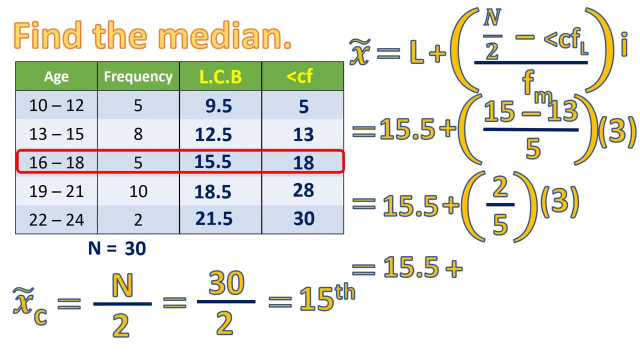 you better multiply first before you divide. So 2 times 3 is 6 and then copy the 5.. So let's continue. We have: the median is equal to. So you compute 6 divided by 5, and then you add it with 15.5, Or you can use your calculator. You will get 16.7 or 16.70, And 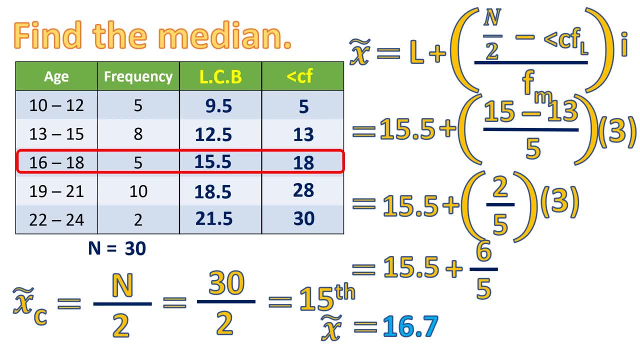 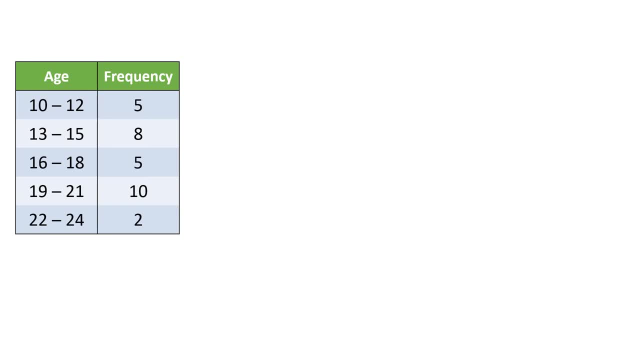 that is the median of this given group data. so let us use the same table, but this time we are going to find the mode of this data. So finding the mode data mode of a group data is kind of different from the ungrouped. finding the mode of ungrouped data. 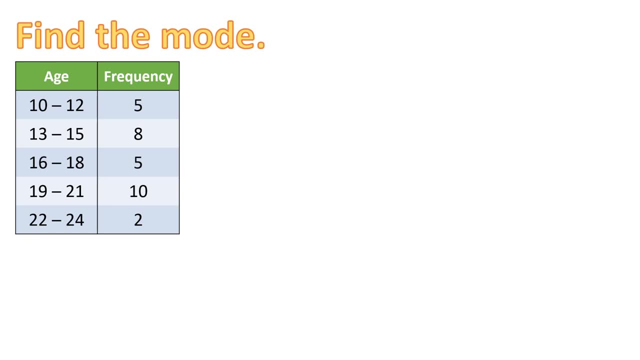 is this simple: just find the most repeating value, while in this group, data is gonna be harder because you don't know what is the most repeating number, because it is by group. it is grouped from 10 to 12, 13 to 15, 16 to 18, 19 to 21 and 22 to 24, and you don't know which of these ages is. 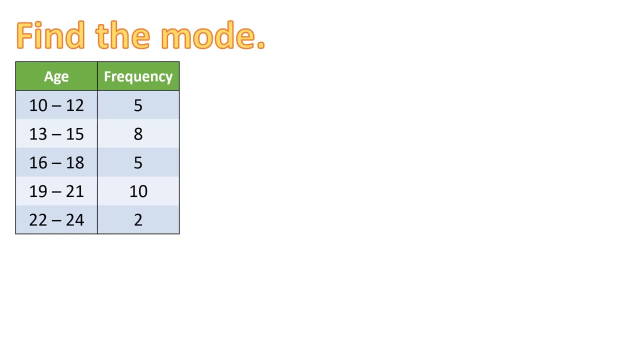 the most repeating, even though you know that there are. most of them are from 19 to 21, but still you don't know which of these three is the most repeating age, and so we're gonna use the formula for mode. so this is the symbol for mode: x, hat, which is equal to l, stands for lower class boundary plus. 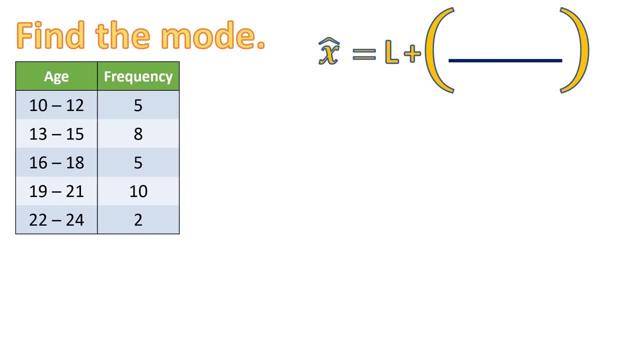 so i have the parenthesis and the ventculum indicating that there is a fraction. so on top is the d1, where is it is the first difference. then copy the d1 plus d2, the second difference, and i will discuss later and you will understand what is the. 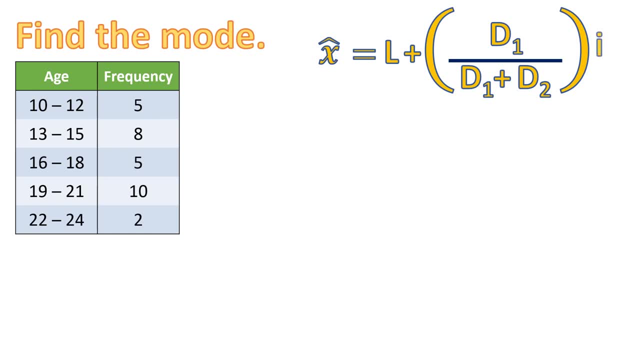 d1 and d2, and all of this will be multiplied by the class interval of class size. and so let us get the lower class boundary, because it is needed in our formula, and we'll just copy the one from the previous slide. it's the lower class boundary, and you know how to. you already know how to find the lower class. 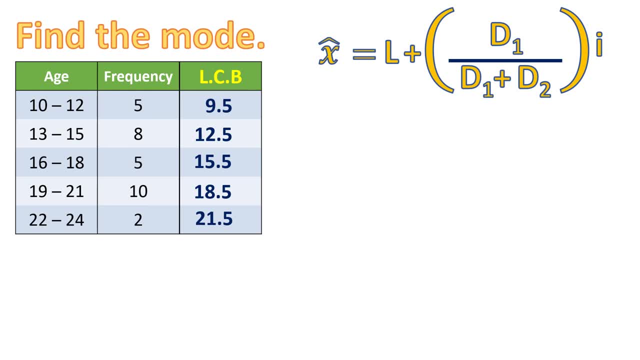 boundary. so now let us subscribe to our channel and we'll see you in the next video. bye, bye, bye, bye. substitute from the formula. now, our problem is: there are many lower class boundaries, so which of this is the one that we are going to substitute? so the same problem with the median. 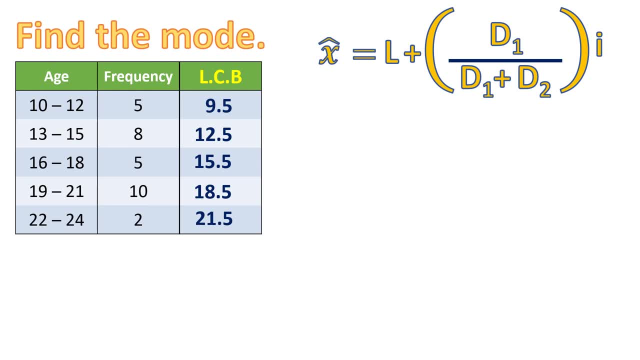 and the same solution. we're going to find our row that we are going to substitute. so in the row in the median class is median class. now the row in the mode is a modal class. so we're going to find the modal class. so how to find the modal class? it is the highest frequency. so in this case, 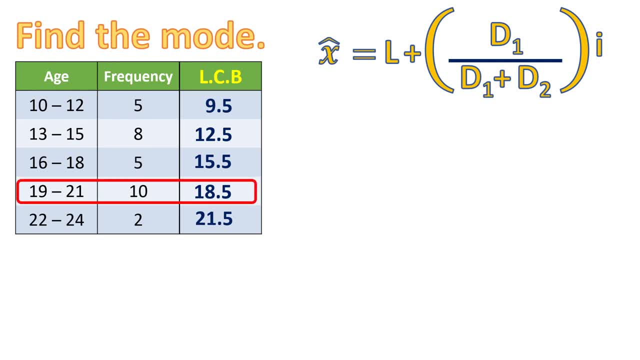 we have a frequency of 10, the row 19 to 21, and this is the modal class. if ever there are two tens in the frequency, meaning there are two- uh, highest frequencies, then that means there are two modal classes and you're going to solve both, because mode can be more than one answer. 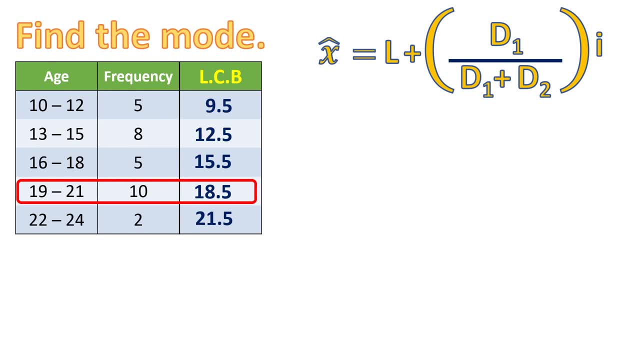 or it can be no more, and so let's substitute, since we already have the modal class. so it is equal to 18.5. that's the lower class boundary plus. so we need the d1. so what is this d1? so d1, the first difference is equal to the frequency of the modal class, which is 10 minus. 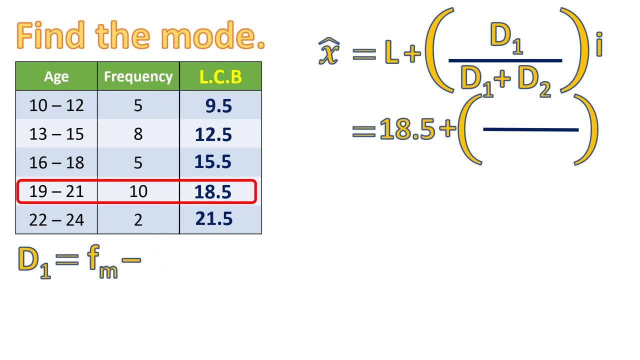 frequency after before the modal class. so frequency before the modal class, before 10, is 5, so it's on top. sometimes the given data is from bottom to top. that means the frequency before the modal class is actually below that. but in this case it is from top to bottom given, so that means the frequency. 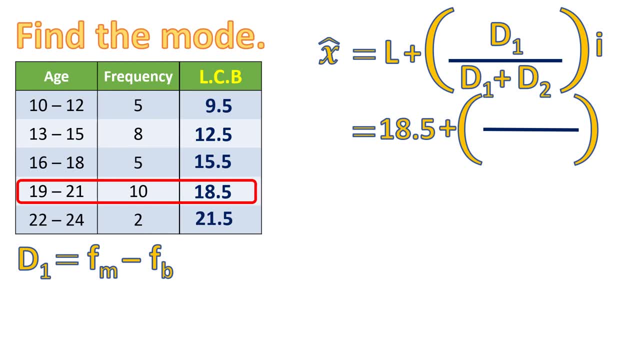 before. the modal class is on top. so this is actually the d1 and we're going to find the difference of these two. so let's substitute: 10 minus 5 is 5, then for d2, for d sub 2, it's equal to frequency of the modal. 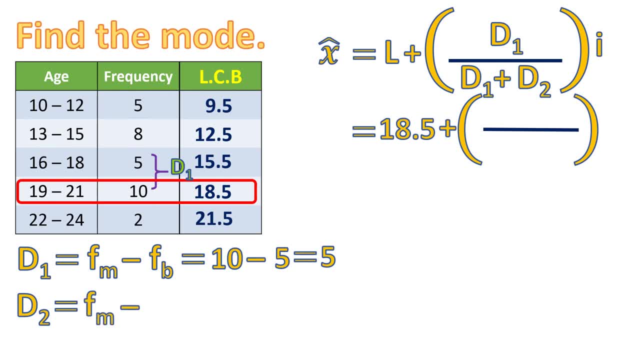 class, which is still the same, 10 minus frequency after the modal class. so it is the after the modal class and then the variable is figure and then we're going toский find the difference. so the same way, if the given is from bottom to top, then frequency after is: 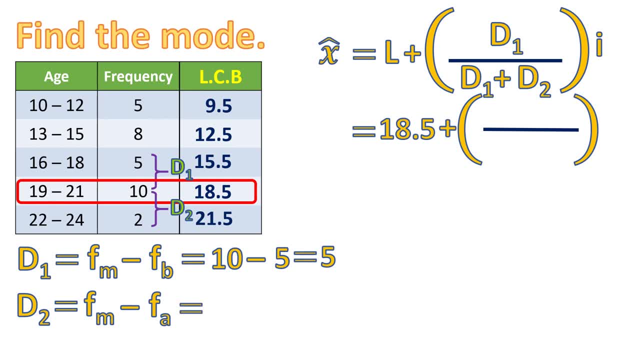 on top of the modal class. so let us substitute. so this is equal to 10 minus 2. so which is equal to that will be substituted in the formula. so d1 is 5, so we'll put both d1s as 5 plus d2 is 8. 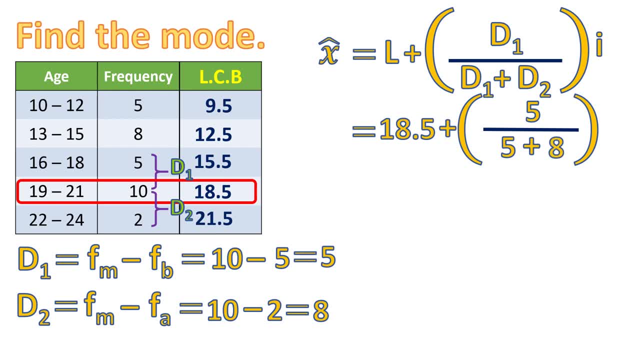 so just allow me to name it and to read it as d1 instead of d sub 1, because it takes it saves time when you read it: d1 instead of d sub 1, d2 as instead of d sub 2, and i is the class size for the class width, so each row is actually having the same. 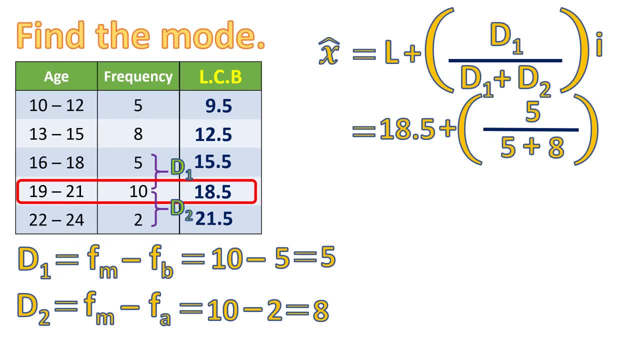 class size: it's 3. 10 to 12 is 3, 13 to 14 is 3, those are the 13, 14 and 15. those are all three, so that's three. it's a class size or the class interval. then let us compute. so let's copy 18.5.